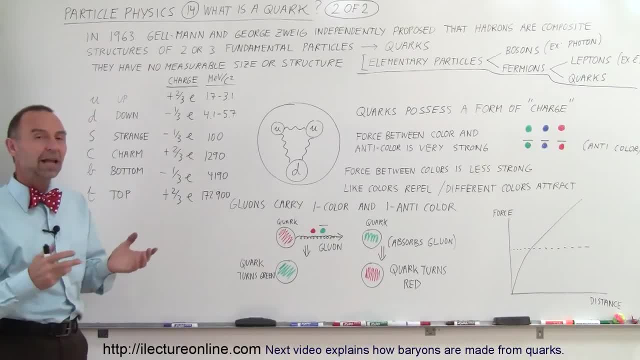 Welcome to Electron Line and to understand quarks a little better now, let's talk a little more about what the forces are and how the forces are created that keep the quarks together inside the nucleon, inside a neutron or proton or any other hadron, and the way that works is, again, that quarks possess. 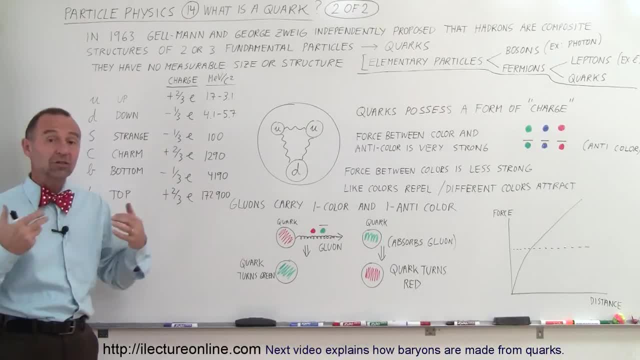 a type of charge. it is not unlike the charge that we're used to positive, negative charges. when they're alike, they repel, when they're opposite, they attract. except with quarks there's more than one. charge is more than a positive, negative. there's three different kinds. and because we didn't have any way to, 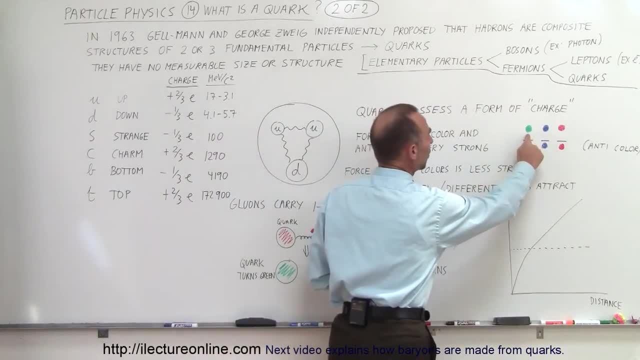 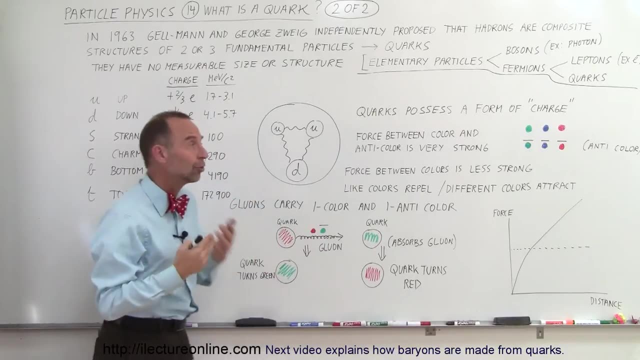 express them? we express them in form of color. so we have what we would call three color charges, and we called them green, blue and red. and again, the color is really not important. just the fact is that there's three different kinds of charges, and we also realize that there is an anti-color charge as well. so for 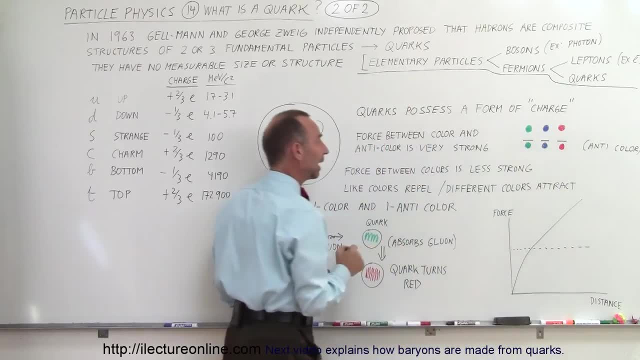 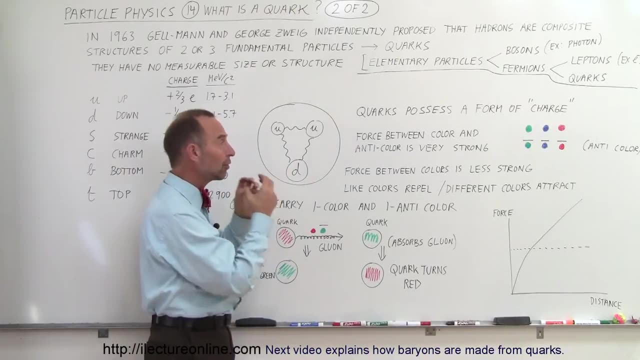 every color charge is an opposing anti-color charge, and what we found was that a color charge and an anti-color charge attract each other very, very strongly. The force of attraction between a color and an anti-color charge is much stronger than the force of attraction repulsion between color charges, And so therefore we can say that the 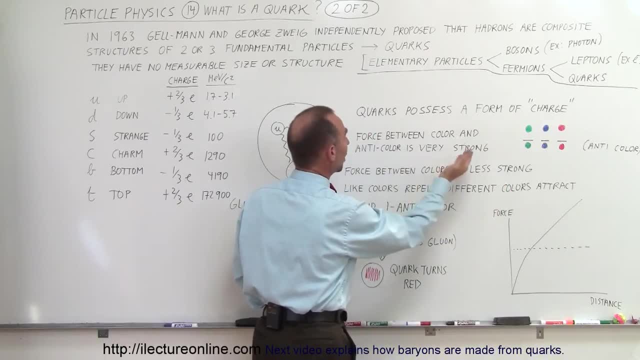 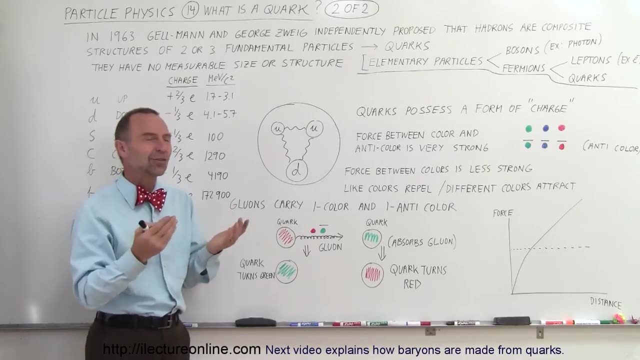 force between colors is less strong than the force between a color and an anti-color. Also, light colors. they repel each other and different colors attract each other. We can't say opposite, because there's nothing that's an opposite. There's just three different kinds. and if they're, 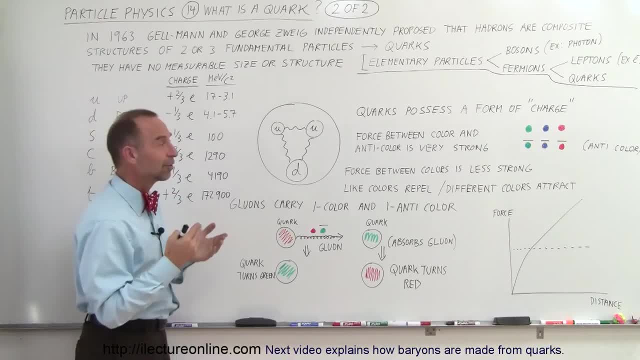 the same, they repel If they're different. for example, a blue will attract to a green and a blue will attract to red, but a green and a green will repel. The way that also works. is that the way the? 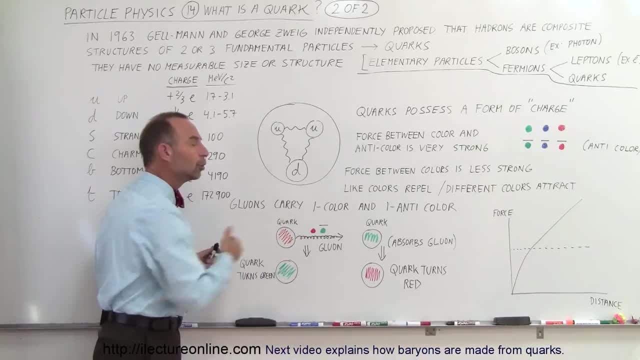 corks interact with each other is through an exchange of gluons. Now that exchange of gluons is a very rapid, continuous exchange. It's not like once in a while a gluon will jump from one cork to another. There's a constant happening. Gluons are going back and forth at very rapid rates and for 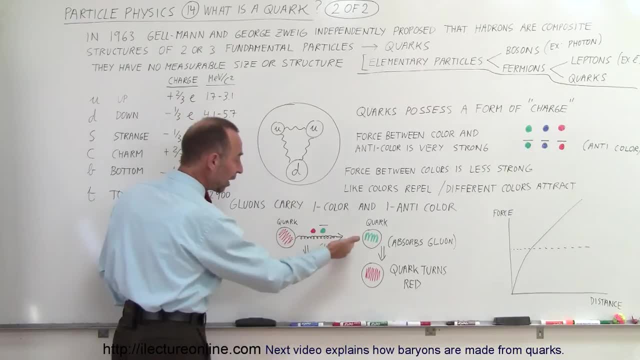 example, when you have a cork that has a red charge sends out a gluon, a gluon will always carry a color charge and an anti-color charge. For example, this gluon could be carrying a red charge and an anti-green charge, And so, by doing that, the cork that then sends out a gluon with 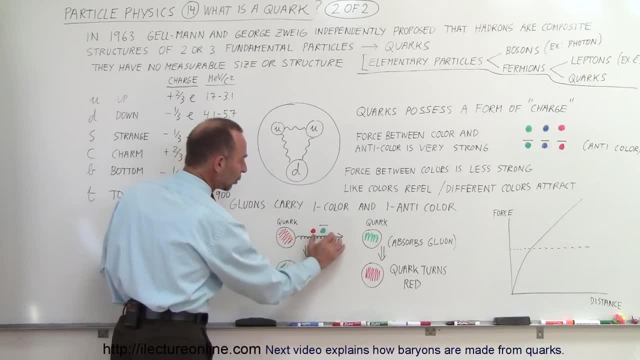 the red charge and the anti-green. the red will then go along with the gluon and the anti-green will cause the cork to then have a red charge. So if you have a cork that has a red charge, you have a green charge and the cork will go from a red charge cork to a green charge cork. 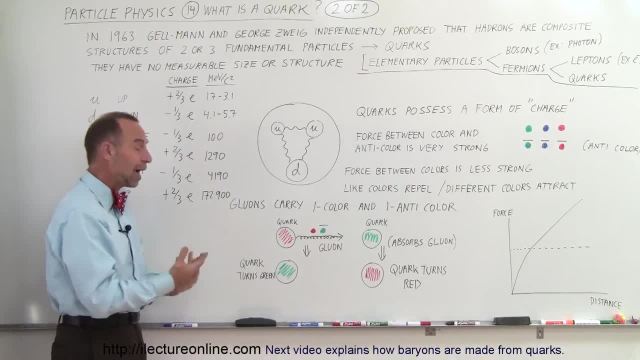 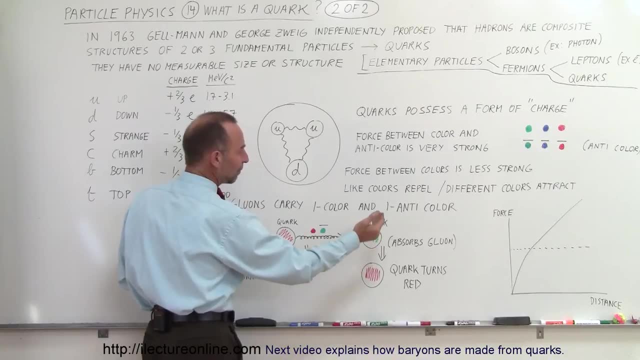 We say that the cork turns green, it doesn't actually turn green. it just now has a green charge associated with it. And then, if let's say, we have a cork that has a green charge on it and the gluon that goes across from this cork to that cork contains a red and an anti-green. 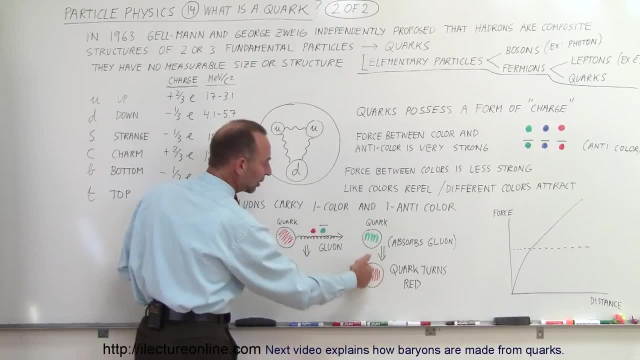 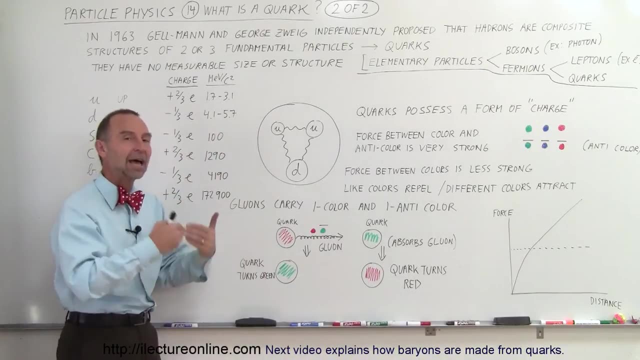 the anti-green will annihilate the green, and the cork will then then will then gain the red charge, and so the cork then turns red. but really what we mean is the cork will now have a red charge to it So before the gluon was sent, since they have different colors. 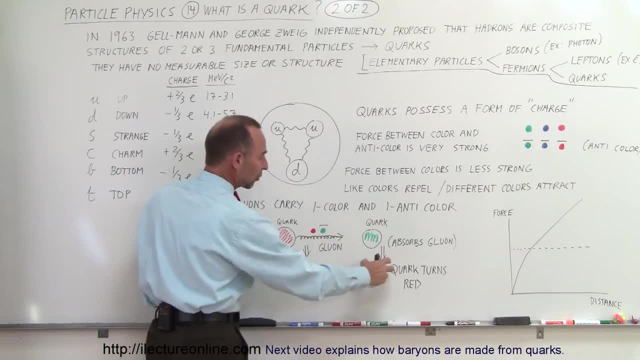 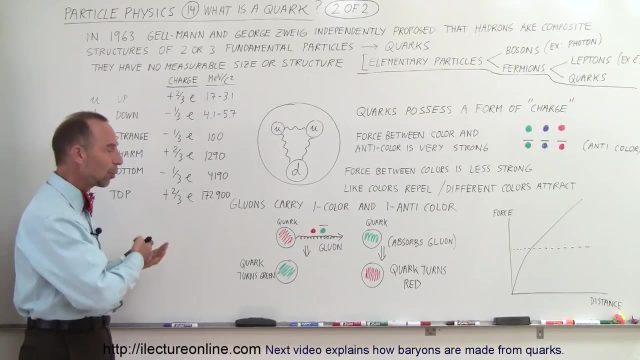 the two corks will attract each other and after the gluon is gone across, the different corks will attract each other again. So you can see that there's this constant balance between the corks having the same color. the corks have a different color Now, while the 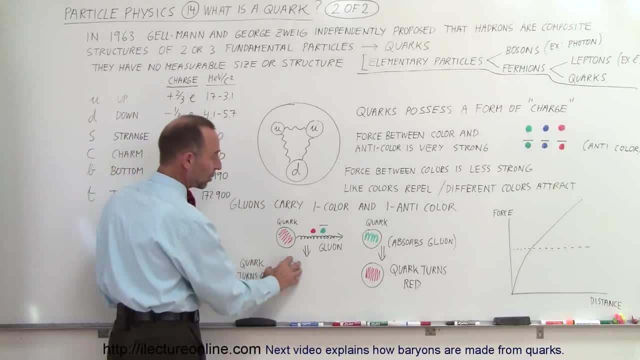 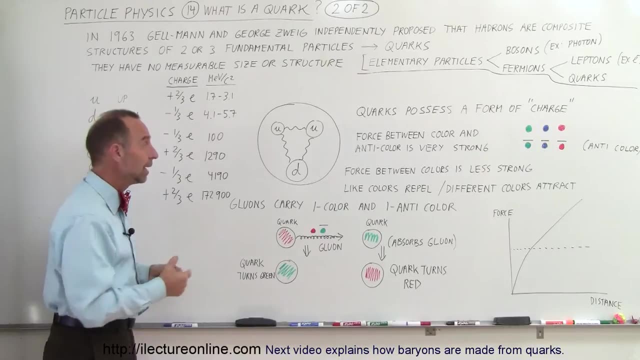 gluon is on its way, this cork will be green. this cork will be green because the gluon is still on its way and, of course, it doesn't take a lot of time. These gluons will travel at the speed of light and the distance between corks is very small. It's smaller than the 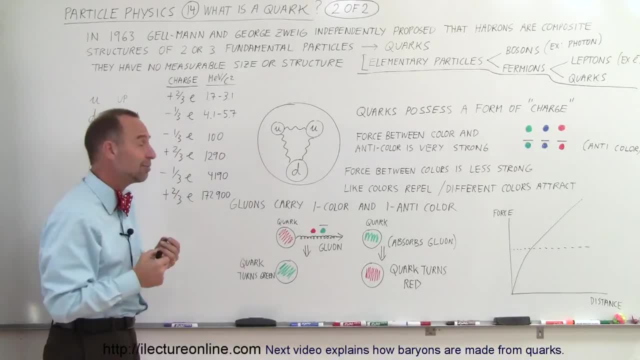 diameter of a nucleon, which is 1 times 10, to the minus 15 meters. so you can imagine the amount of time that the gluon spends traveling from one cork to another is extremely small. but during that very small amount of time those two corks now have the same color and 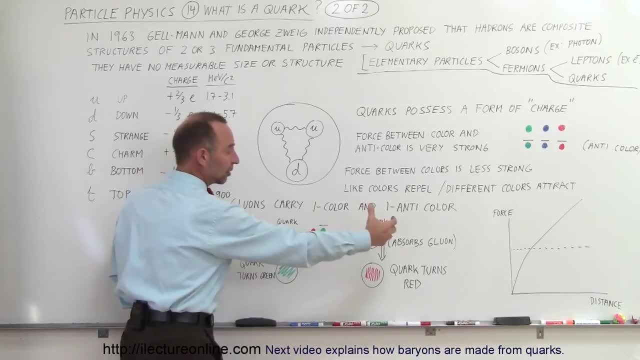 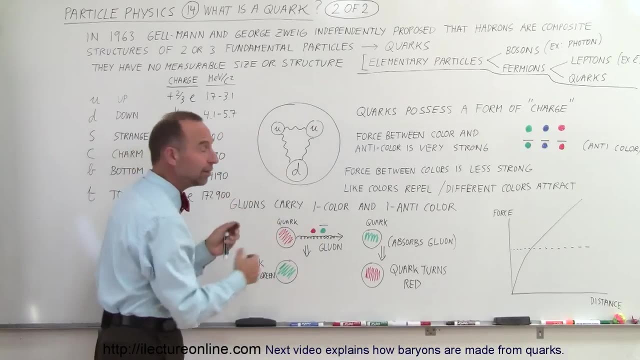 they repel each other, So the corks will move farther apart. then, when they attract each other, they'll start moving closer apart, and so there seems to be this constant balance. There's a constant balance between corks as these gluons go around. Of course, if you. 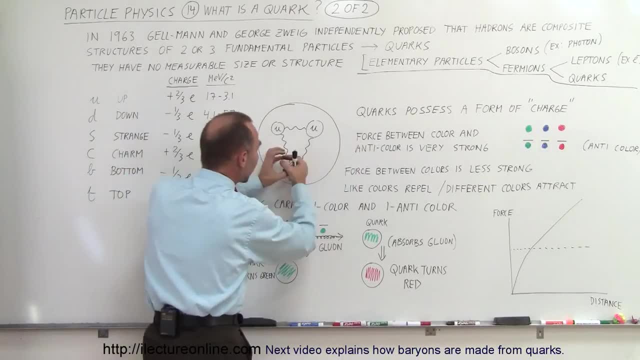 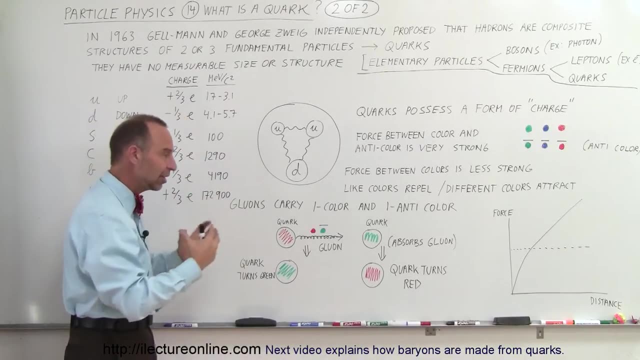 didn't have. if you had a static situation, then the corks would either attract each other and collide, or they repel each other and disappear. so that can happen, We have to have them in a certain balancing act, so to speak, and therefore this constant exchange. 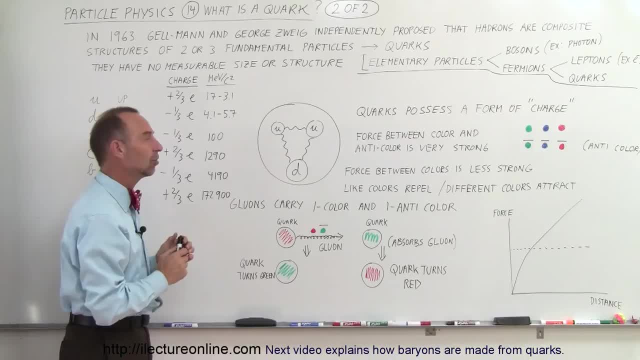 of gluons makes sure that these corks will remain at certain distances. What we also found was, as the corks move farther apart, the exchange of the gluons becomes more rapid and the force of attraction then becomes greater, As we see in here, as the distance 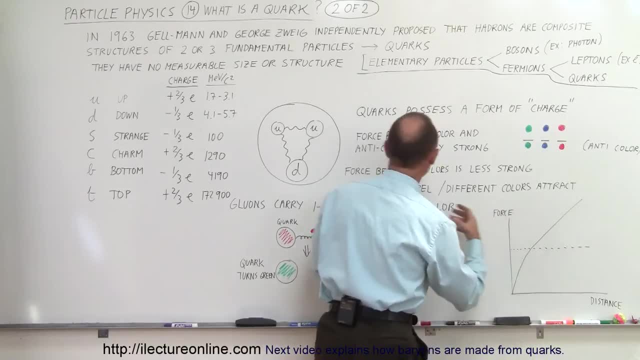 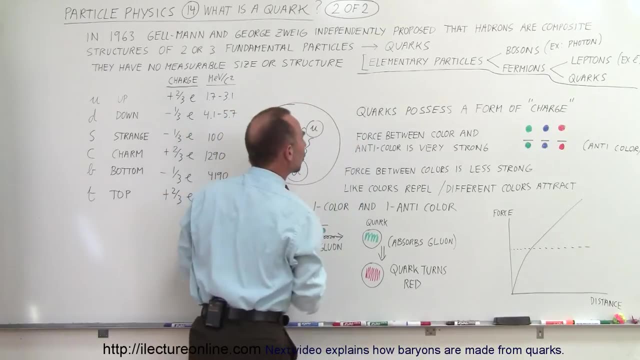 between corks increases, the force between them increases, and so that increase in force prevents the corks from moving too far out and leaving the boundaries of the nucleon, or the proton, or neutron, as we want to call them. All right, so hopefully that gives you. 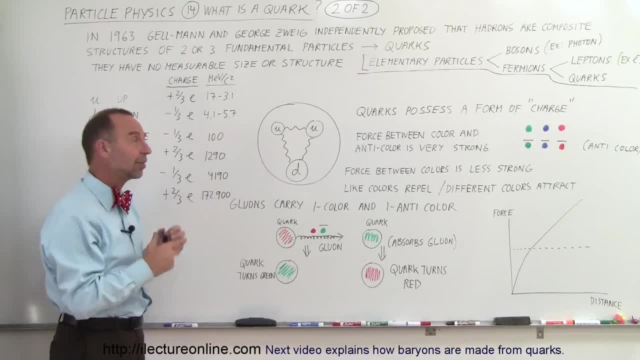 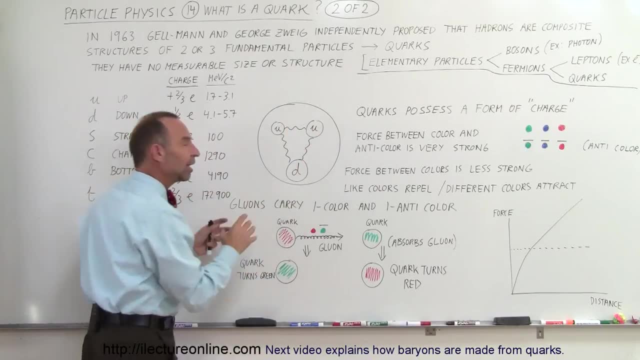 a really good feel of how these corks actually balance in. there Again, the vast majority of the mass of the corks is the mass of the gluon. The vast majority of the mass of the nucleons is not made up of the static mass of the corks. 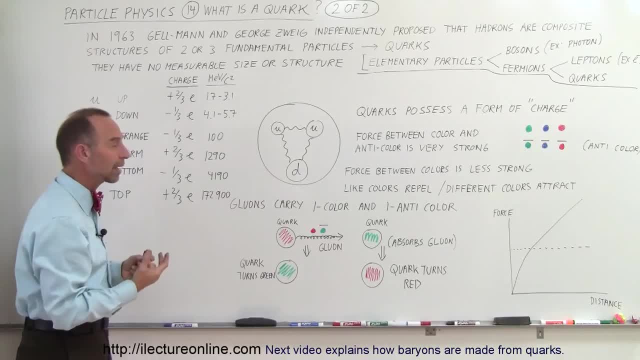 but it's made up of the energy exchange that happens when the gluons go back and forward. Remember, gluons, just like photons, contain a lot of energy and therefore that energy then makes up the mass of the nucleons. So that gives you, hopefully, a better idea of 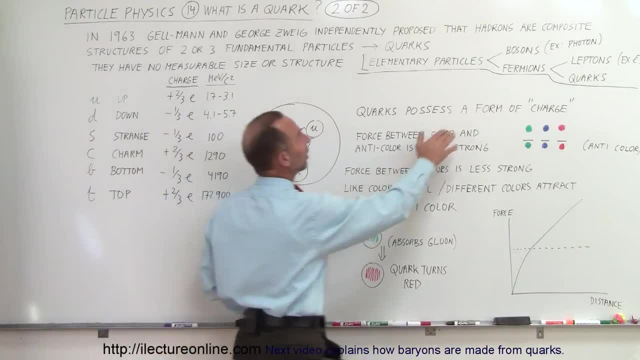 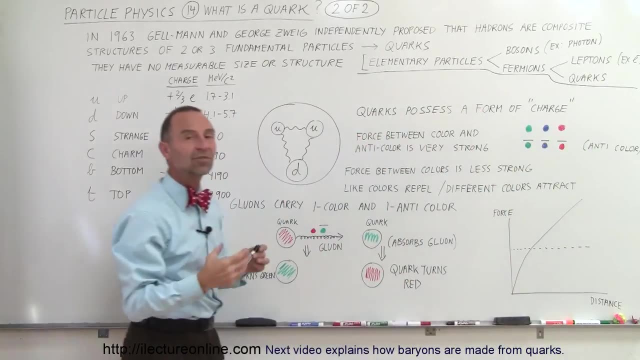 what corks are? Corks are these elementary particles. They're actually part of the fermions which make up leptons like the electron, and then, of course, the corks is a separate set under the basic elementary particles. We don't think that corks are subdividable. 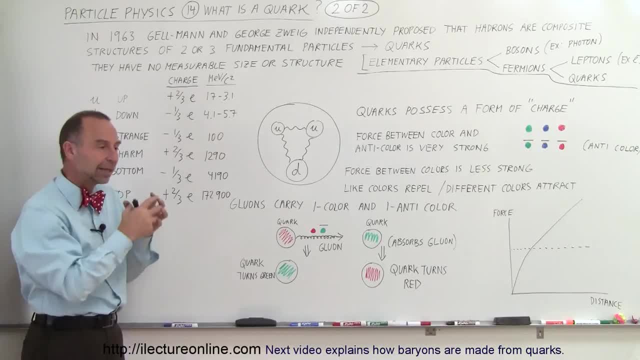 so we don't think that they're structured to corks, We don't think that they're subdividable, that they're individual units without any basic dimension as we know it, or I should say dimension, because they do have dimension but any basic structure to them, Just like. 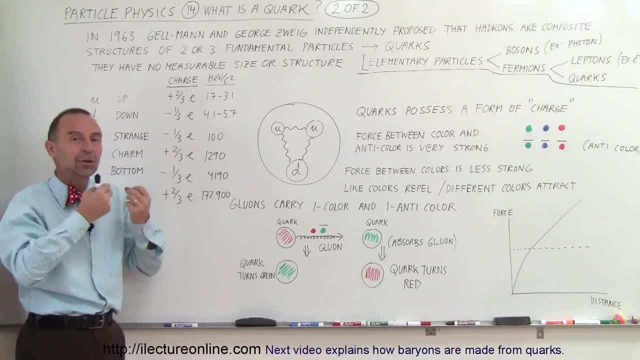 an electron seems to be like a point object. corks tend to be looked at as point object. Something interesting to note, though, that some corks have an enormous amount of mass, and I realized in the previous video- I didn't have these numbers correct because I moved. 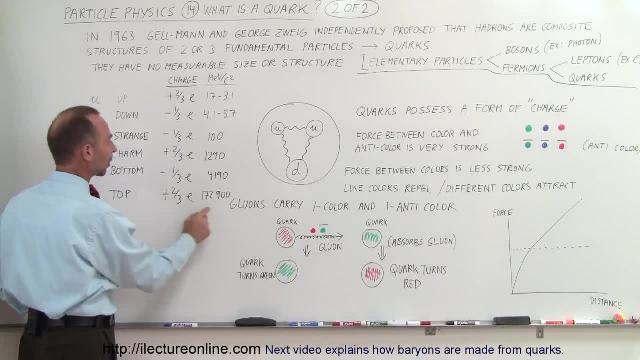 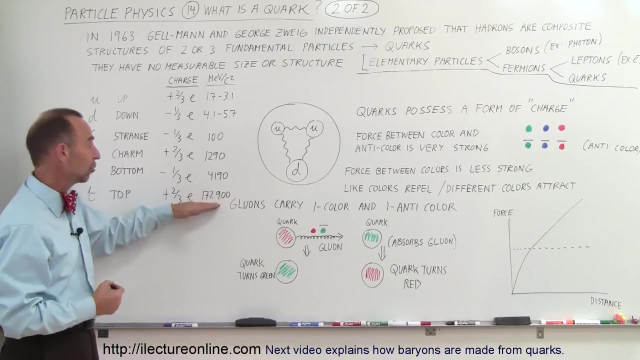 these around a little bit, but realizing that if you take a look at the top cork, it has the mass of roughly- let's see here roughly- 175, 180 times the mass of a neutron or a proton. so some corks have an enormous amount of mass associated with them. Notice that.